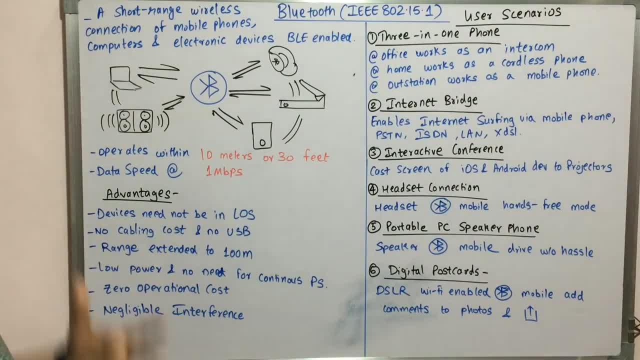 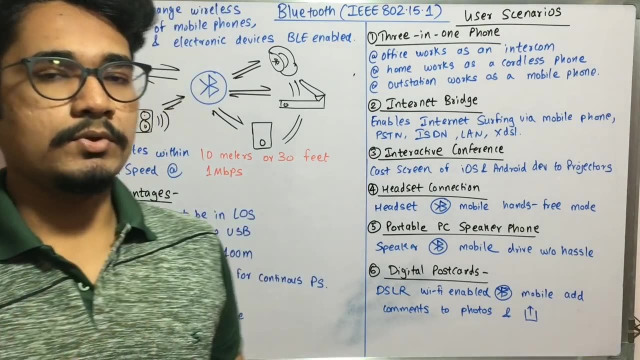 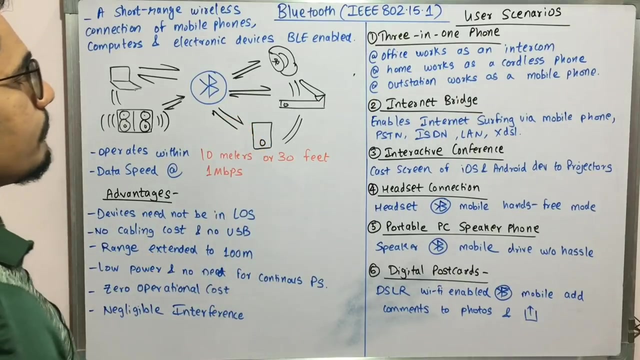 is Bluetooth, So it is a low power consuming technology and it operates within a short range and it provides wireless connection to mobile phones, computers and electronic devices which are Bluetooth enabled. So there can be a number of devices which are not Bluetooth enabled but in Bluetooth it demands that each of these devices should be Bluetooth enabled. So this can be considered of a fitness tracker, like this MI Band 3, and it can be a scanner. This can be a smartphone. These are some speakers and this is a laptop. 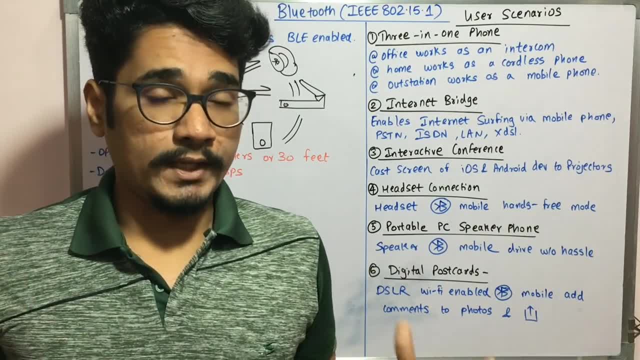 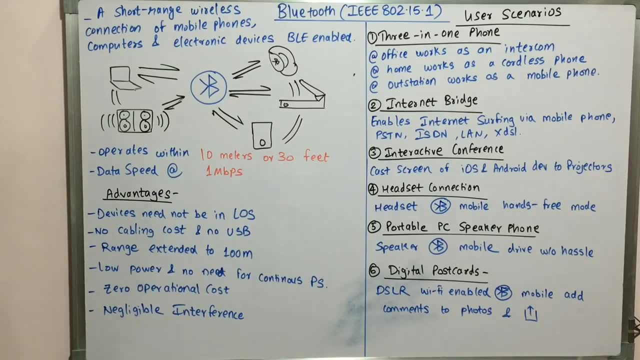 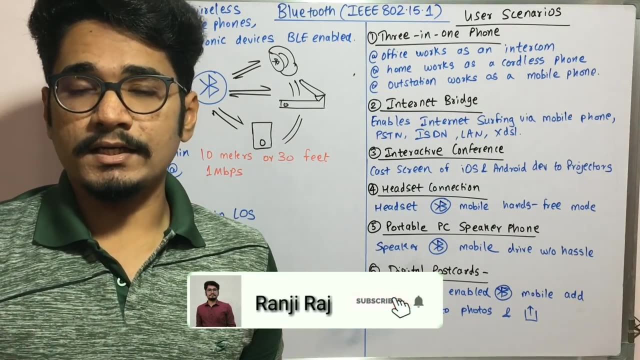 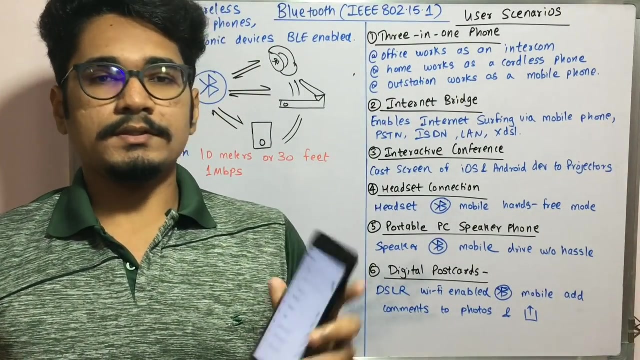 So in most of all these devices you have this Bluetooth enabled. So let's begin. So this Bluetooth operates within a range of 10 meters to 30 feet and it have a data speed of about 1 Mbps means a data transfer, or the file transfer which you do, It is done at a rate of 1 Mbps. Now in this video, I have just bought my smartphone, So in this you can have this. This is an Android panel of how a Bluetooth basically looks like. 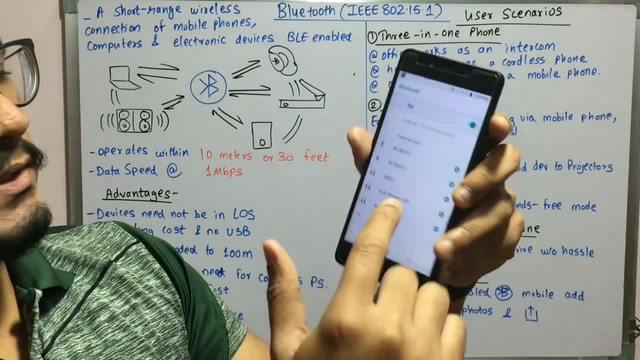 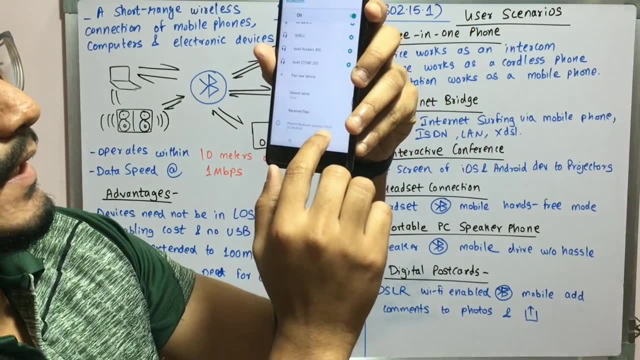 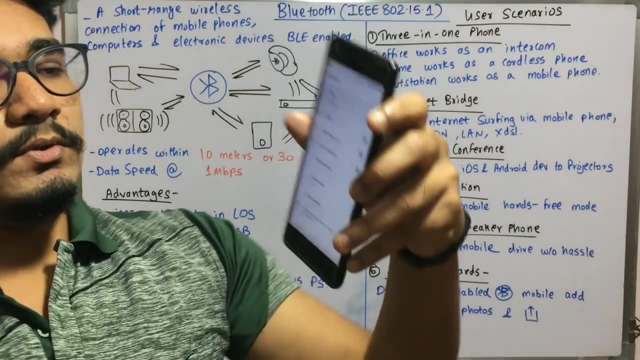 have this various devices, like you have paired devices. then you have the device name as well as you have the phone's bluetooth address. here that is something d86c022800 and 05. so this you can see. so this is the bluetooth panel in android how it looks like. so these are the various devices. 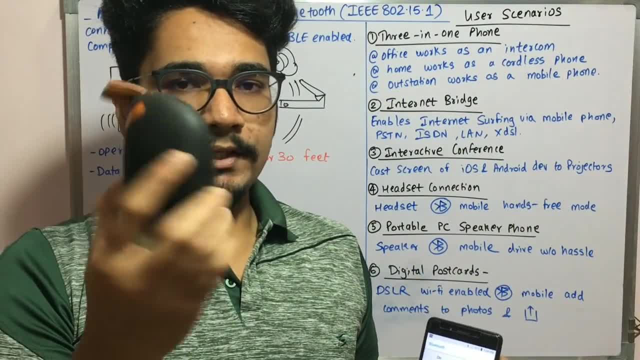 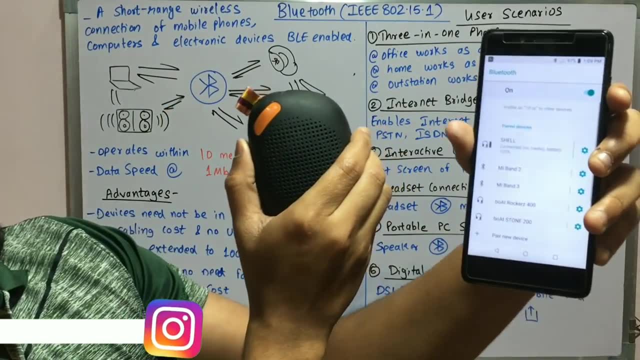 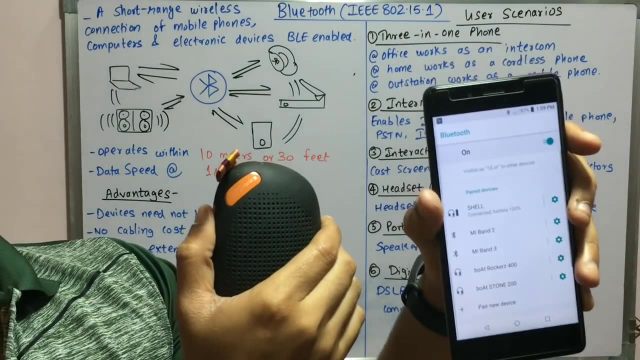 so this is my bluetooth speaker, so i'll just connect. first i'll just on this device bluetooth mode, next i'll just move into this distance so you can see the device is connected and so it will show the battery percentage as well. so this does not necessarily mean that the devices should be. 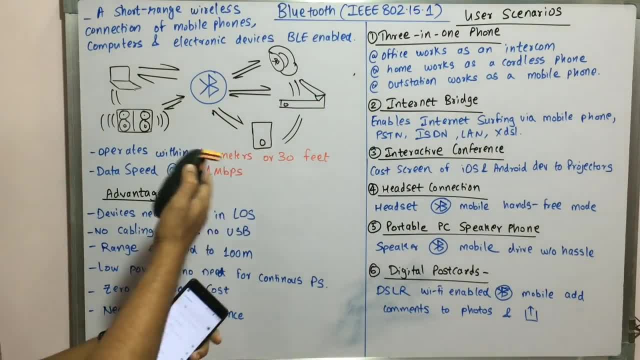 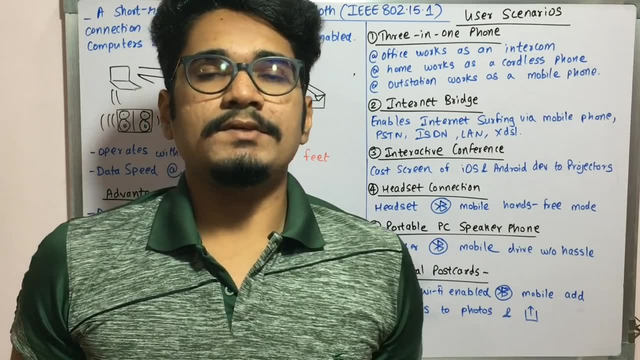 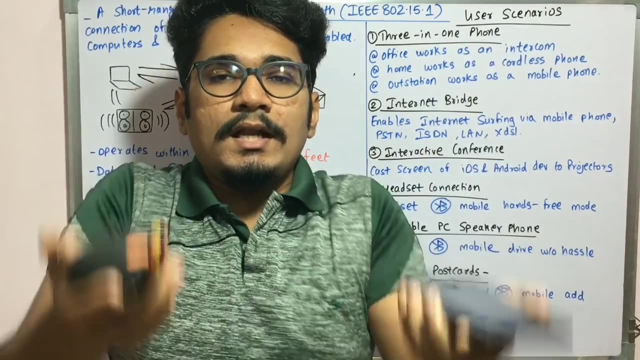 very nearby, or it can be up to this distance, or 10 meters or 30 feet, if it is within this proximity, and be paired. and so this device does not necessarily require that they should be facing each other. they can be at a long distance or they can be even lying down on some table or some on. 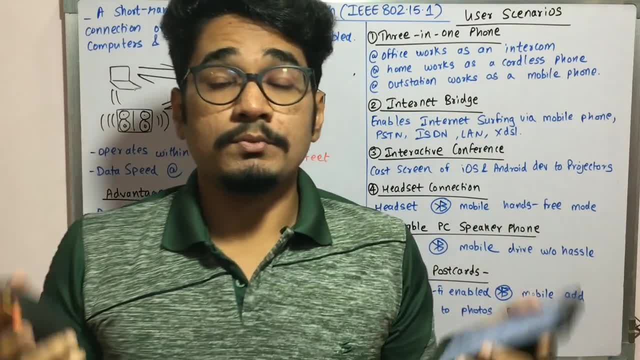 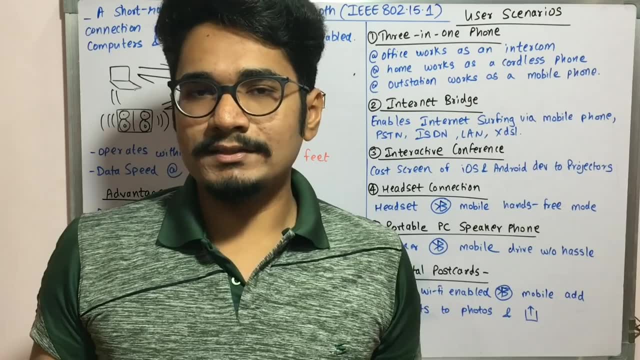 solid objects, so there is no necessary that these devices should be actually facing each other like in other technologies, like in nfc or in other zigbee protocols and all. you need these devices facing each other and so there is some topology where these devices are connected, so in bluetooth. 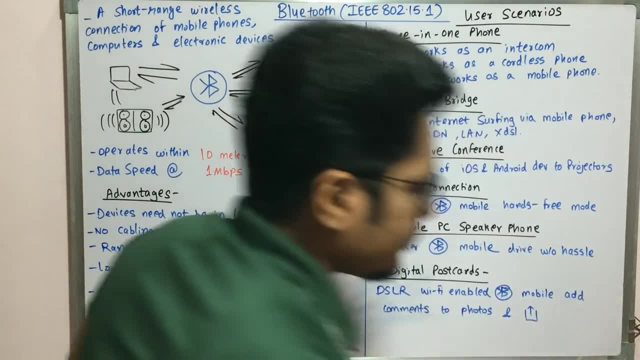 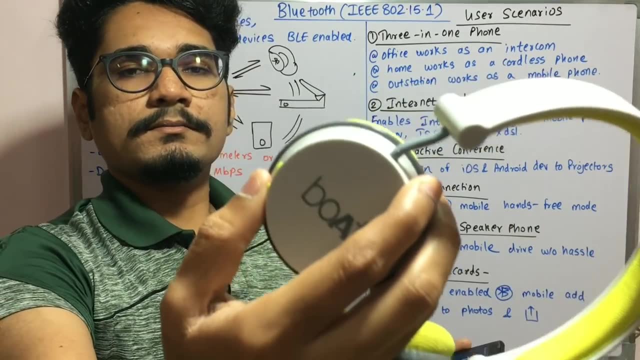 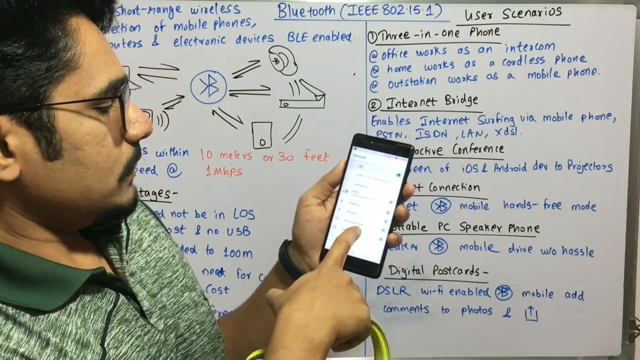 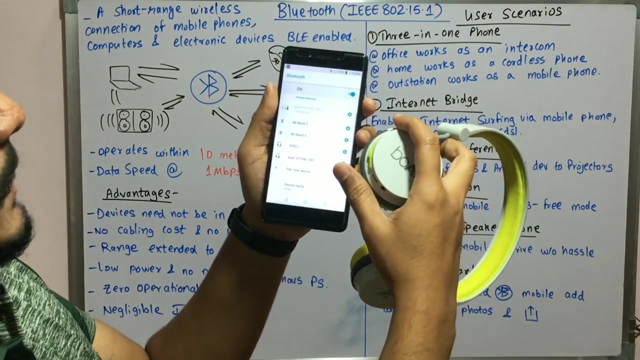 you don't have all those hazards. next, i have this uh bluetooth uh headphone, or my headset. so, uh, this also is bluetooth enabled. so this is a boat headset. now i'll just connect this device. so you have boat rockers. 400 device is ready to pair. so, uh, it will just connect to. 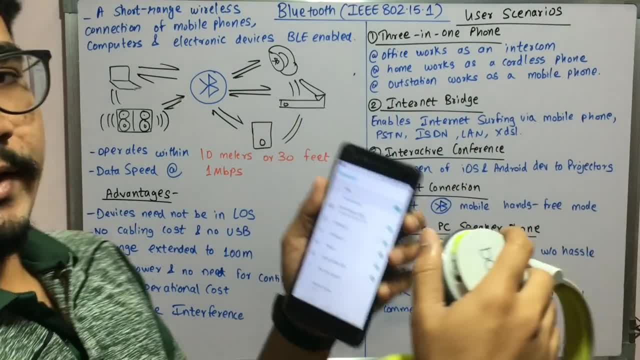 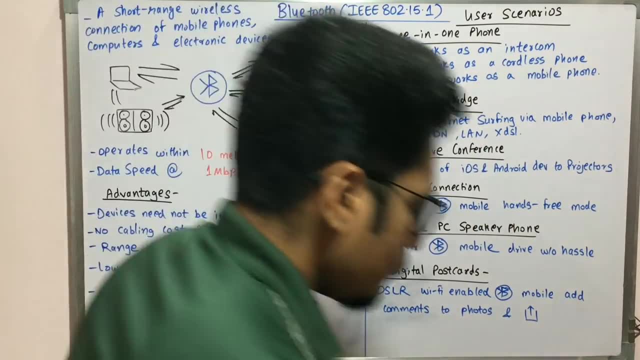 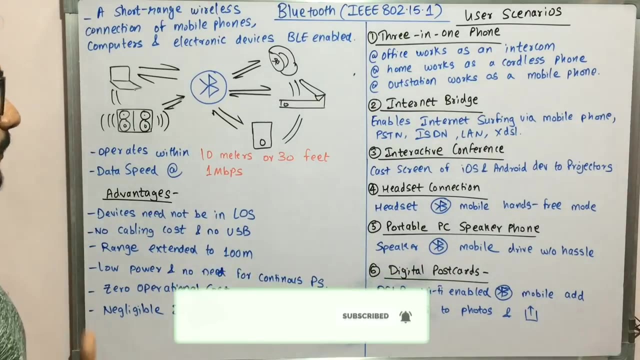 boat rockers: 400, so you can see the battery percentage. so, as you can uh see this devices be at a larger distance, even at smaller distances they can be paired, and so, uh, we move on to the advantages of what bluetooth basically is. so the devices need not be in the ls, ls means the 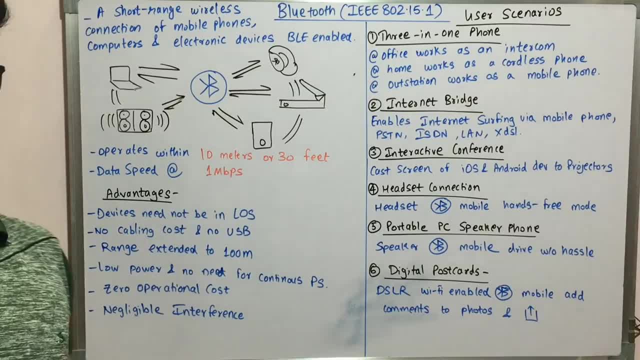 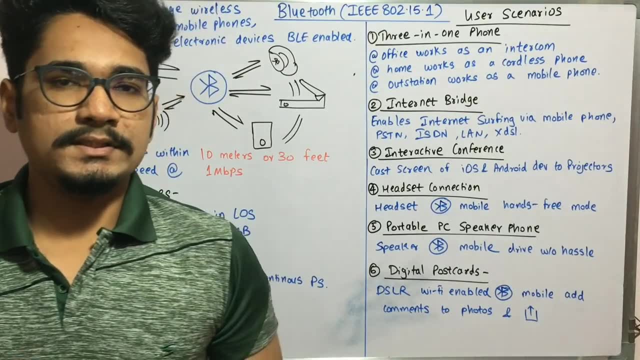 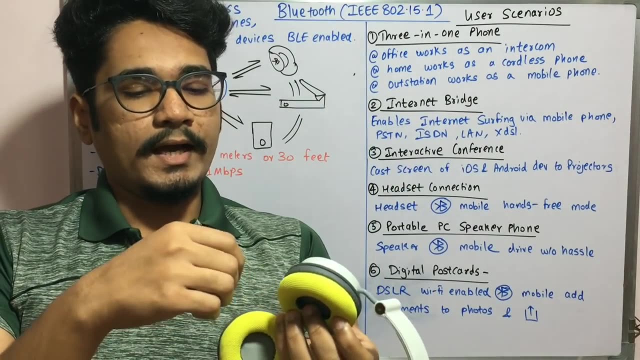 line of sight. they can be at uh the specified range, or they can be in the nearby vicinity also, and no cabling cost or no usb. since you see how these devices are basically connected, you don't need a physical wire. obviously, with this uh, i had got a wire, but i 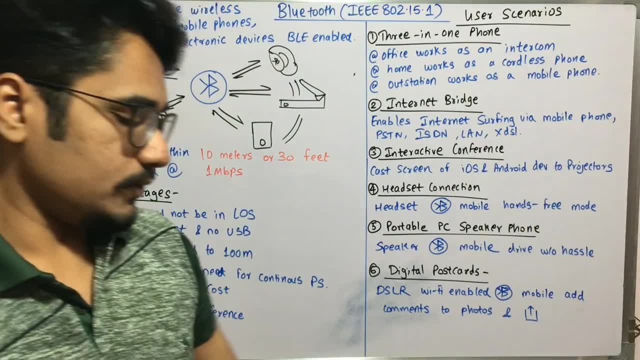 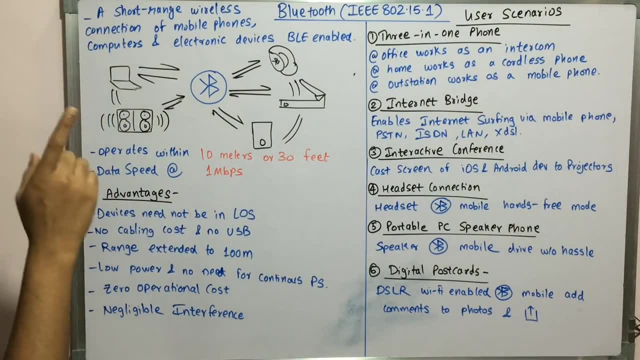 did not need any wired connection in order to access that, so that i've showed the practical demonstration. and no cabling cost was there in this and so, uh, mainly no usb was there, so you don't have a w usb setup in this and the range is extended to over 100 meters so you can have. 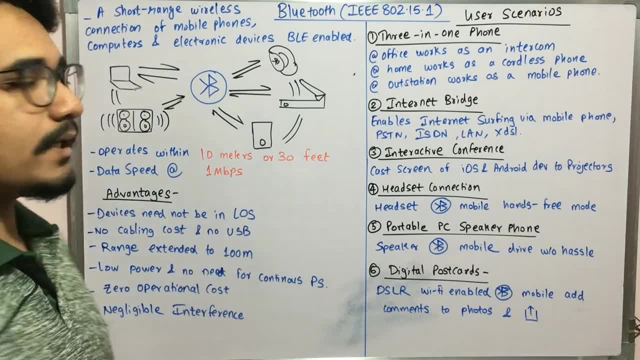 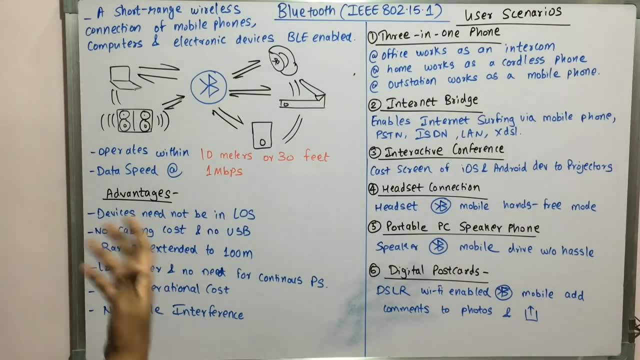 uh bluetooth extenders where you can just extend this 10 meter range to even 100 meters and it has low power consuming and it does not need any continuous power supply for it. so you can see the battery percentage, how much you can use. it depends on the device you are using. it depends on the 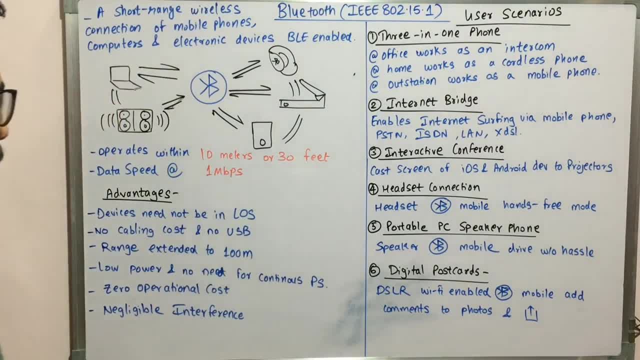 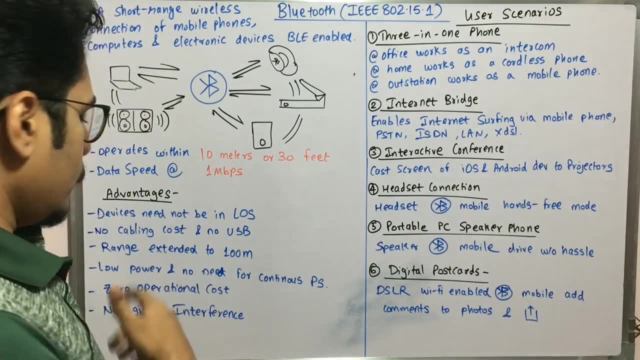 how much it utilizes of your storage battery of your smartphone and there is no operational cost. so the operational cost associated with it is very low and a negligible interface. so you saw i have connected two devices, like i had my headset as well as my speaker, so there is no kind of 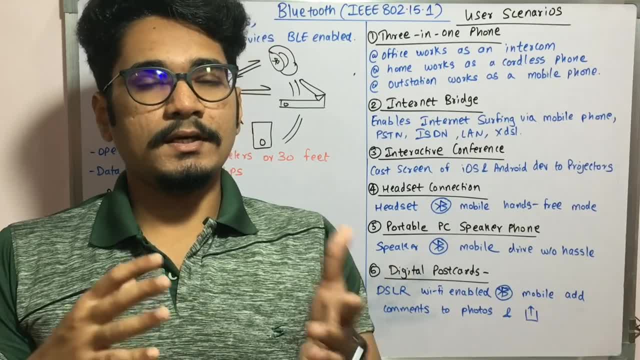 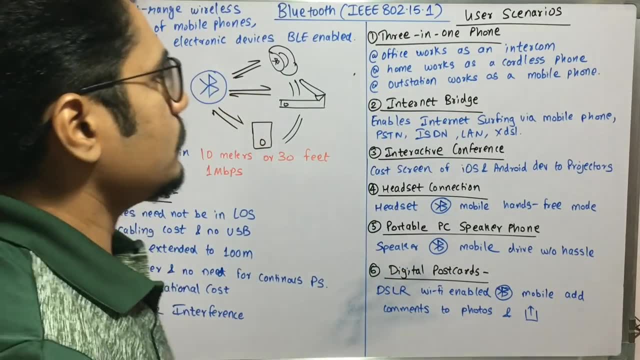 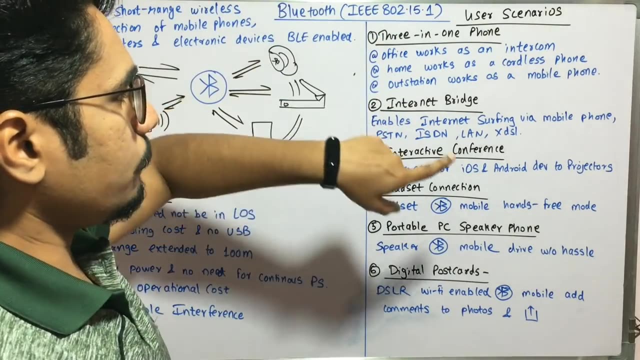 interference between the connections. so this is a major advantage of bluetooth. next we move on to some of the user scenarios where bluetooth are used in the real world applications. so to begin with, very first, one has bluetooth connection, so bluetooth connection is very important for bluetooth. we have the three in one phone, so this can be considered as your phone at your office. it can be. 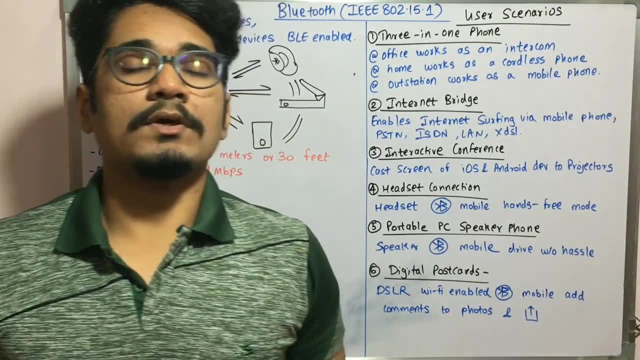 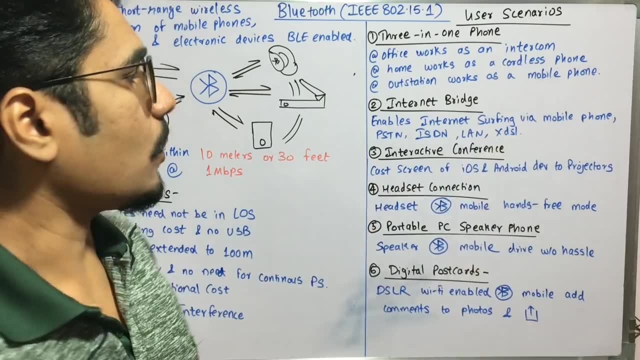 made to work as an intercom where you can get to know what all persons are, who all are coming to meet you. so there you can make use of your smartphone with bluetooth enabled as to function as an intercom, and at home it works as a cordless phone where you can just roam around and do the 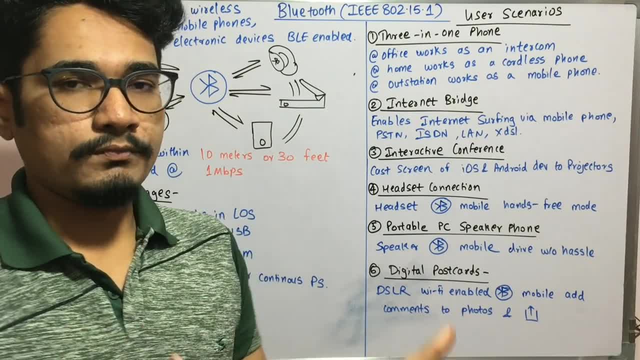 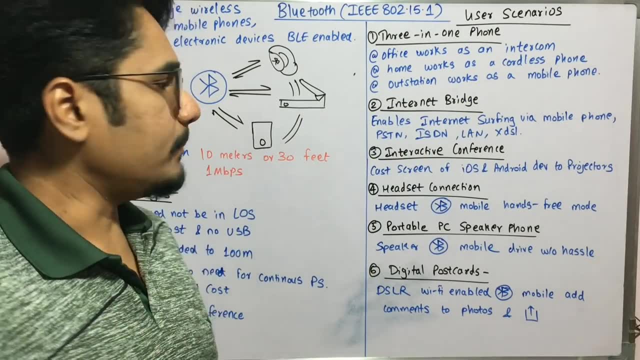 communication and an outstation. if you are not at home, not at office, then an outstation. when you roam outside, then it can function as a mobile phone. next, we have the three in one phone, so this is the internet bridge, so it enables internet surfing via mobile phone, like you have, if you. 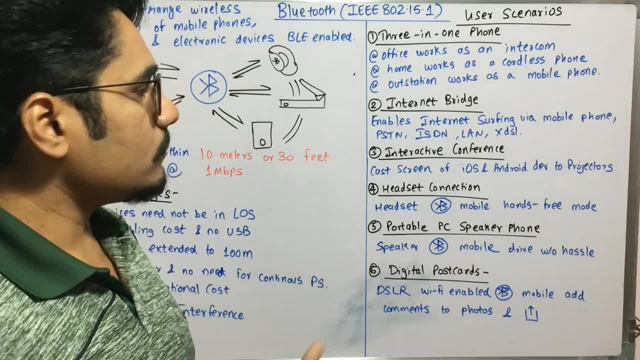 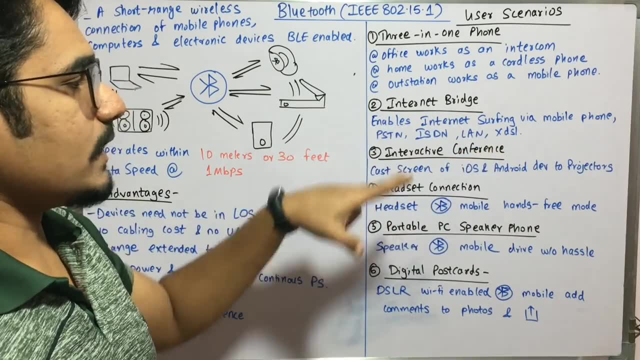 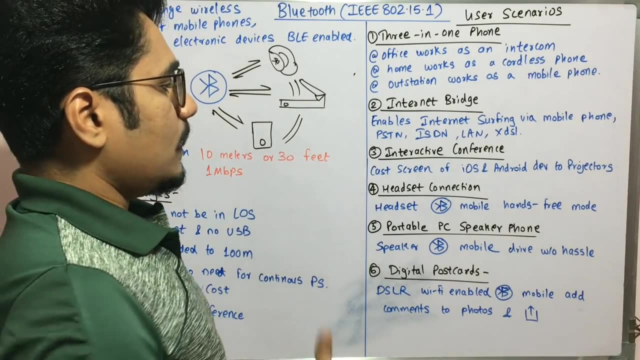 don't have a wi-fi access, or if you don't have a net access, then also you can do the internet access with the help of pstn and isdn, then lan, xdsl, so all these technologies, when you just connect with the bluetooth, you can do the internet surfing. next you have the interactive conference, so it 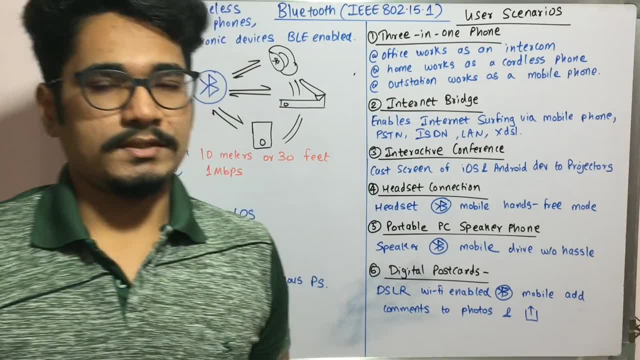 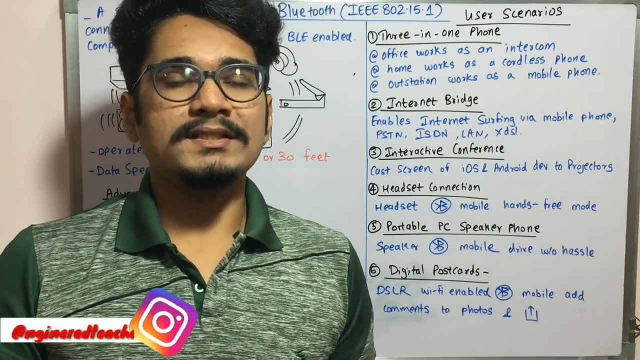 basically cast screens of an ios or android device into projectors. so in windows also you have this option. so whatever your android screen is or the whatever your home page is, that gets projected to a projector or some screen kept at some distance. so that's basically the feature which is provided. 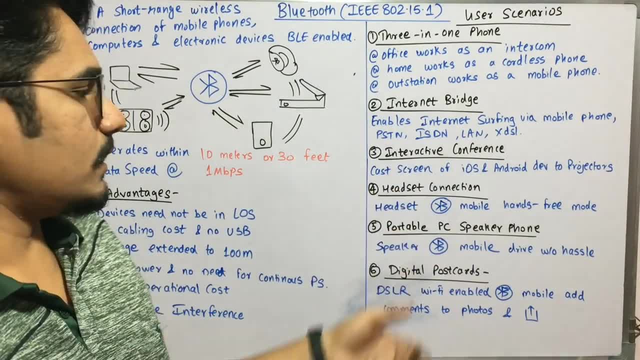 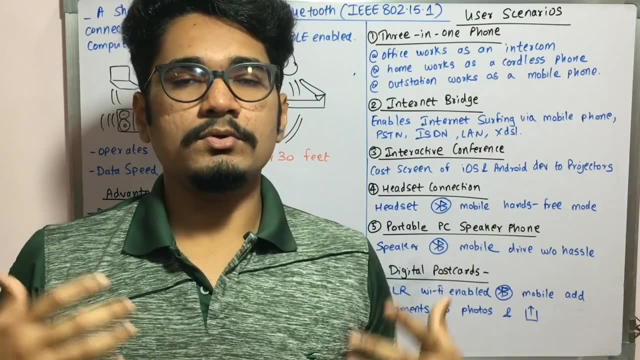 by the bluetooth, and then you have the headset connection that i demonstrated in this, so you have hands-free mode. so whatever you do, or if you just plug on to this device with the help of bluetooth, you can do any other activity without any hassle. and then you have the portable pc speaker phone. 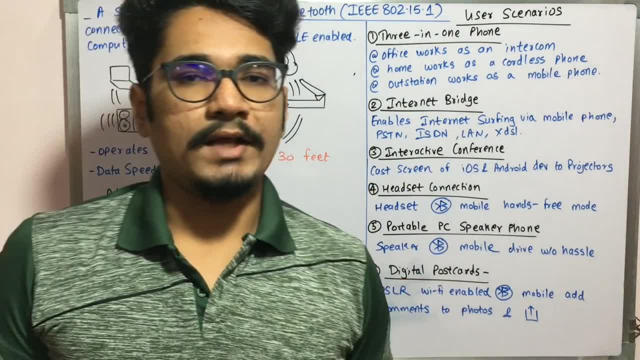 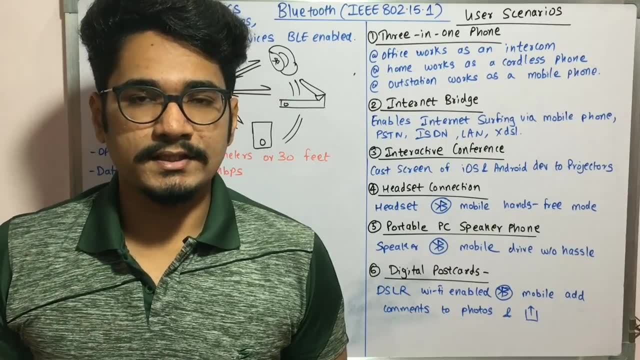 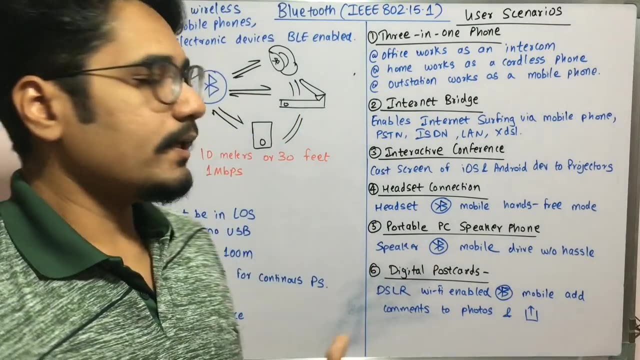 that was also i shown you, but this isn't in case of driving. suppose, consider you are driving and if you get a call from some person, then what you can do is you can do the hands-free setup in your phone connected to the bluetooth enabled setup of your cabinet of your car, and then you can drive without any hassle and you can also speak. 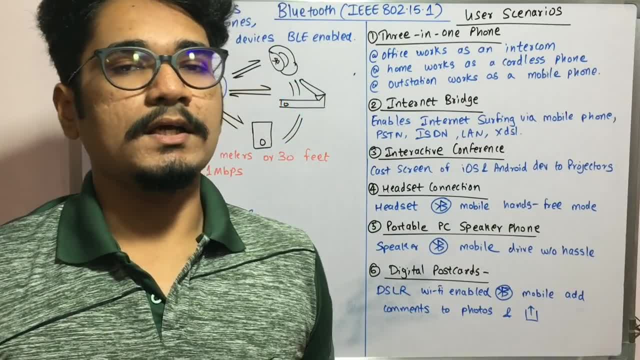 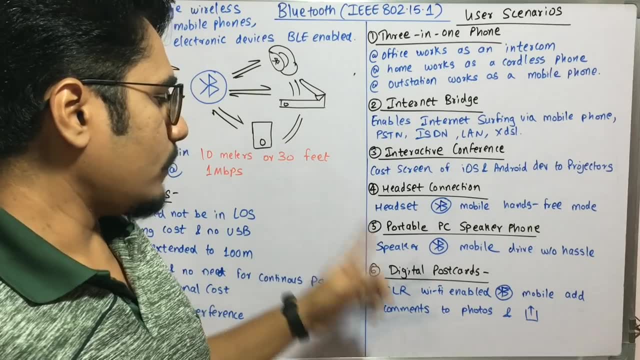 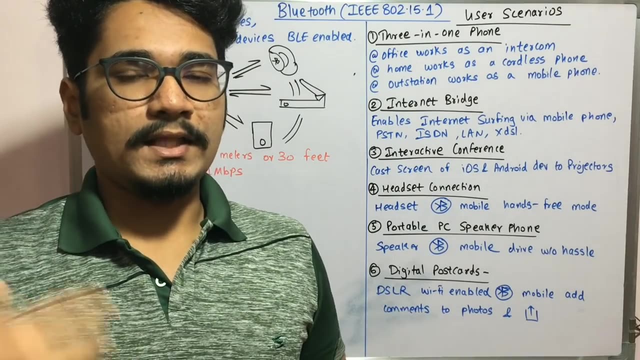 while you are driving, so that will minimize the cause of accidents, which are mainly happened in this kind of activity. and then there is something called as the digital postcard, so you have this reflex most commonly called as dslr cameras. so some dslr cameras with higher ranges are wi-fi enabled.